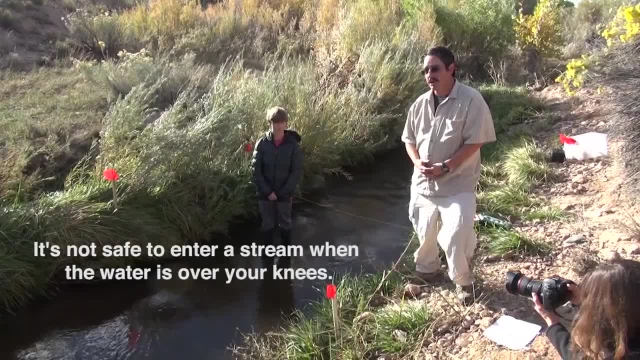 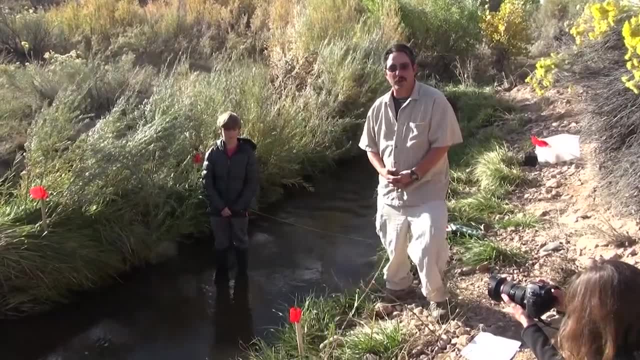 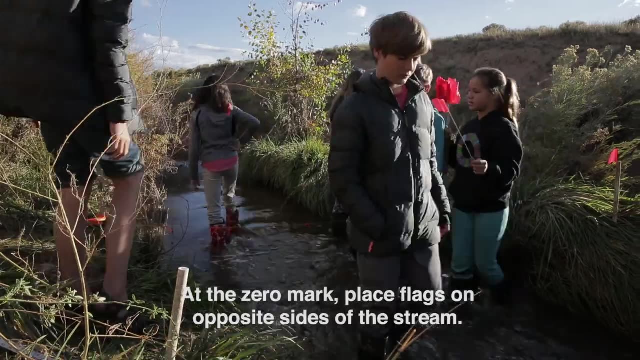 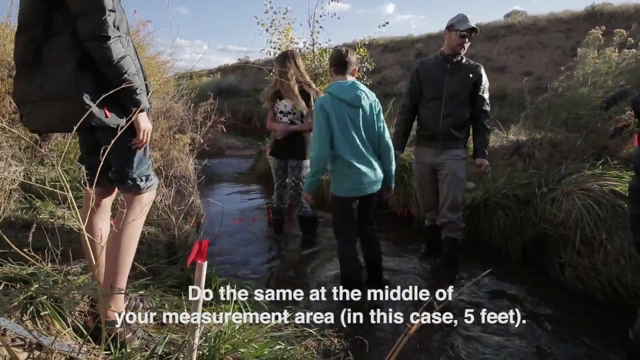 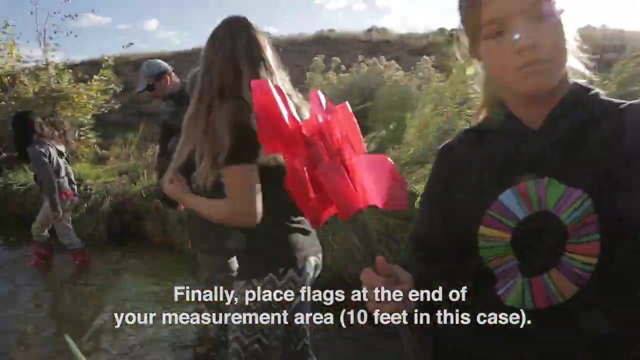 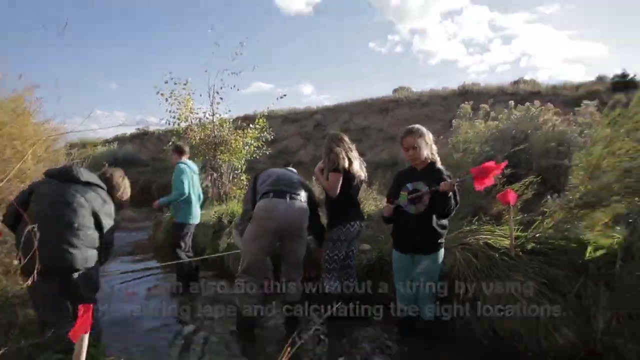 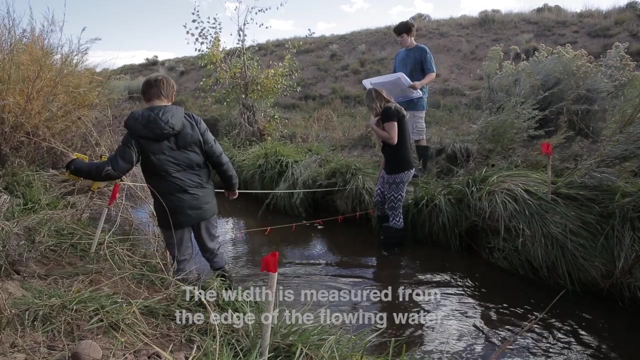 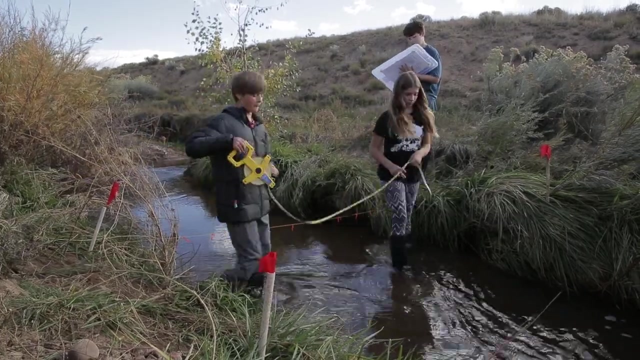 that the water may be too deep or dangerous for you to go in, and often times this can occur during flood conditions, so do not monitor flows during flood. We're measuring width: 6.5. 6.5?? Yep, 6.4. 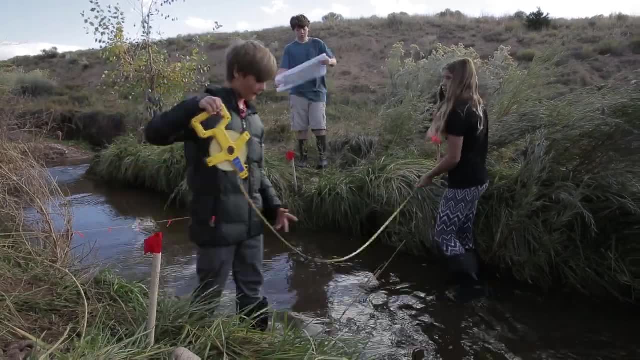 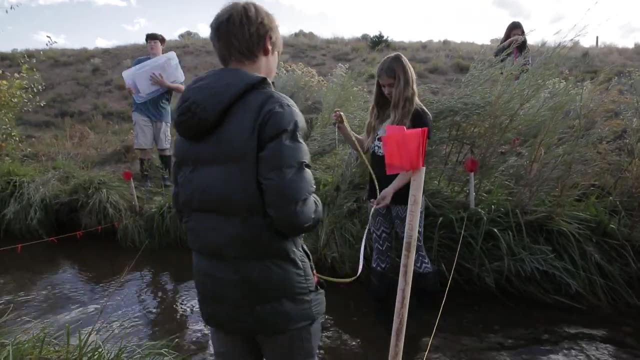 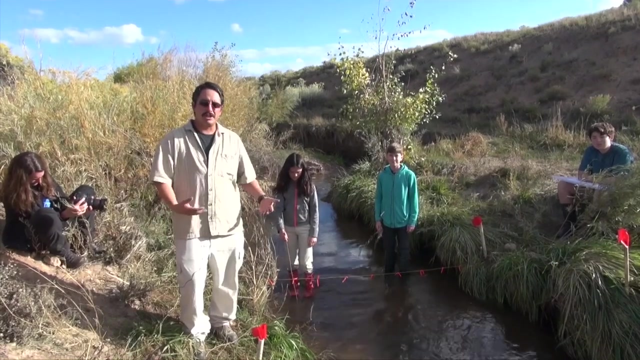 6.4? Yep, 6.2, 6.2? Yes, We are now measuring depth. In order to measure depth, we've evenly divided the stream channel based on the width. In order to do this, we divide the width by the length. 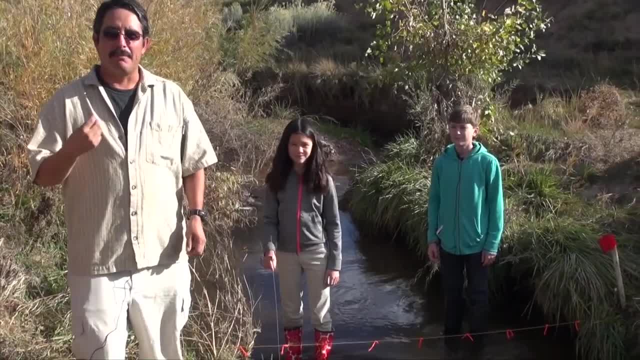 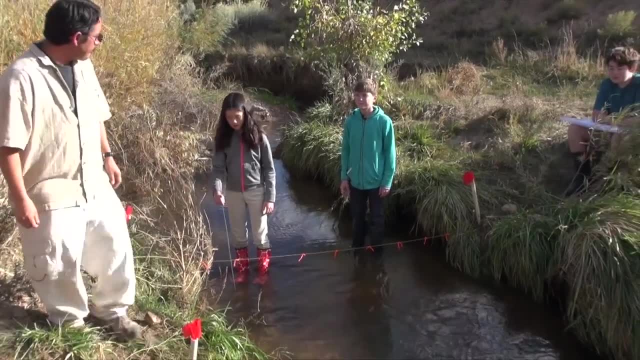 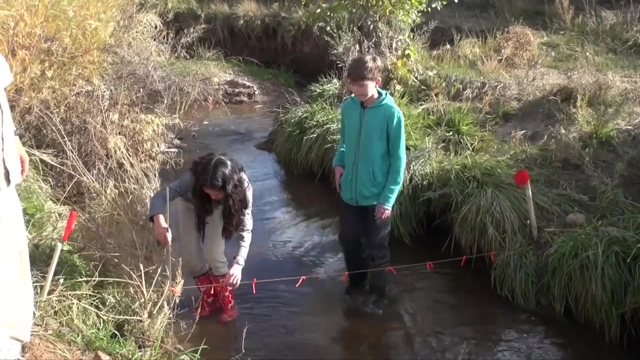 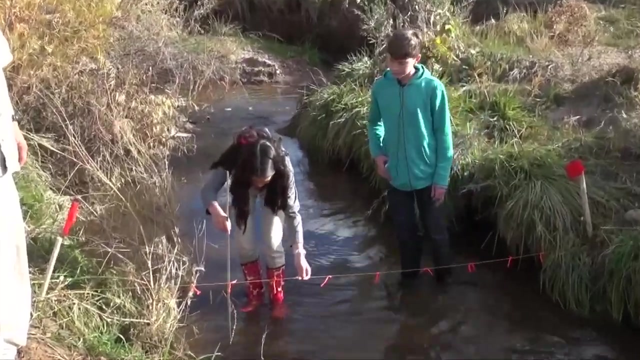 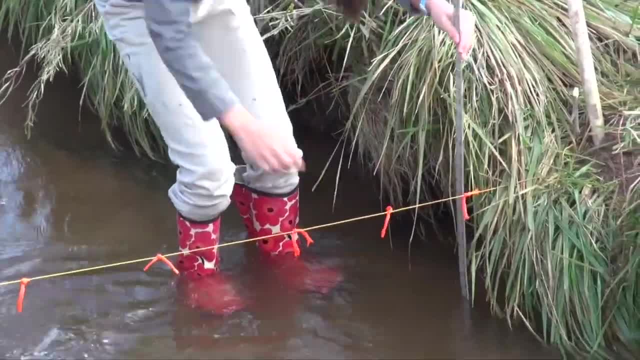 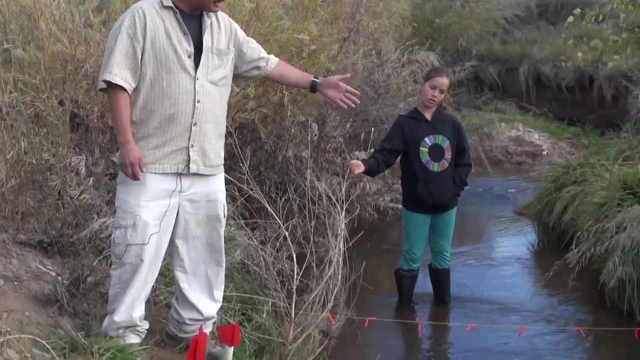 6. 6. 7.5, 7.5, 7.5, 7.5, 7.5, 6. 6.. In order to develop a velocity, we will be floating in orange through the six center sections of the stream channel here. 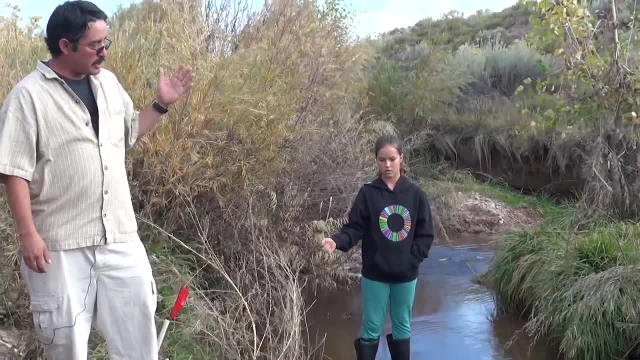 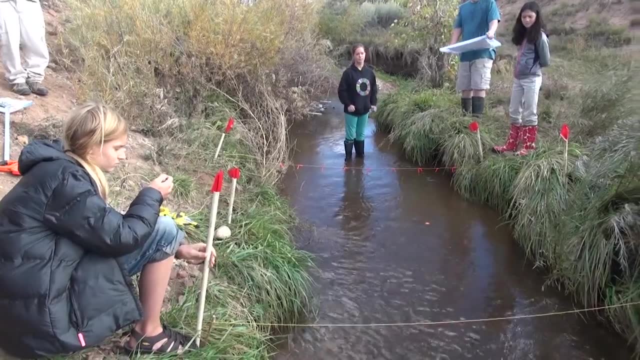 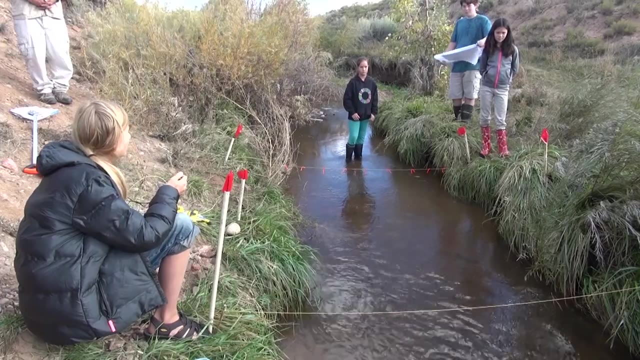 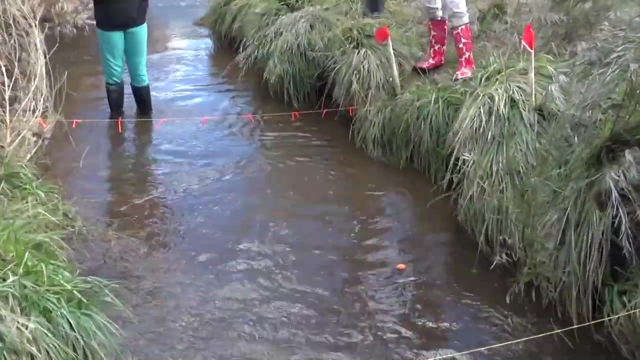 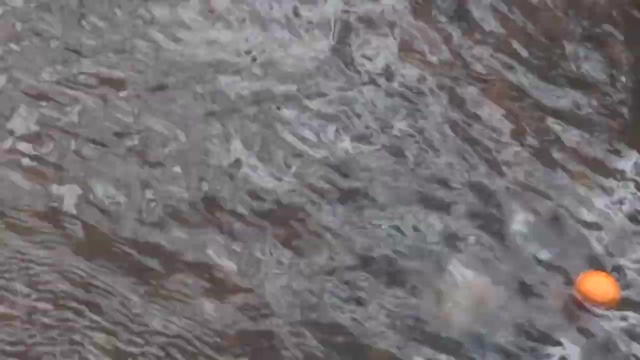 Students will time how long it takes the orange to get from the start to the finish line. Start Stop. 8.75- 8.75? Yes, 7.4- 7.4? Yes, Alright, Start Stop.